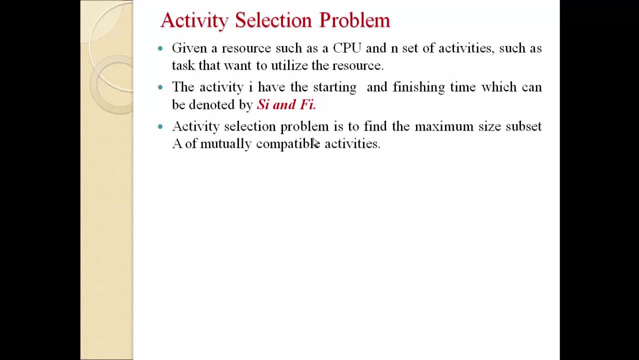 of mutually compatible activities. so one activity must be compatible with another activity so that we can execute both the activity. so we have to identify, we have to maximize the total size of our capital air in that we are storing, uh, all the compatible activities. so first of all, try to 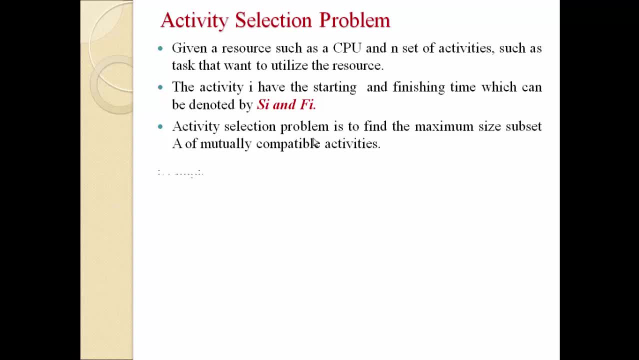 understand what is compatible activities are. just take an example. suppose we have a list of activities, one, then a one activity, a two activity, a three activity, up to a eleven activity. total eleven activities are there as we discuss. every activity has some starting time and finish time, so activity. 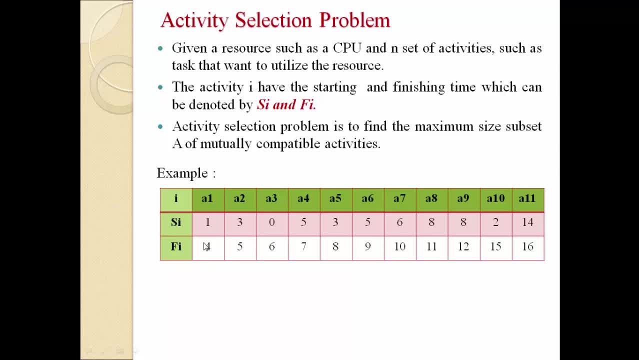 one has starting time one and ending time is four. activity two has a starting time three and ending time, that is a finish time, is five. activity three has a starting time zero and finish time is six. so likewise, every activity has some starting time and a fixed finish time. 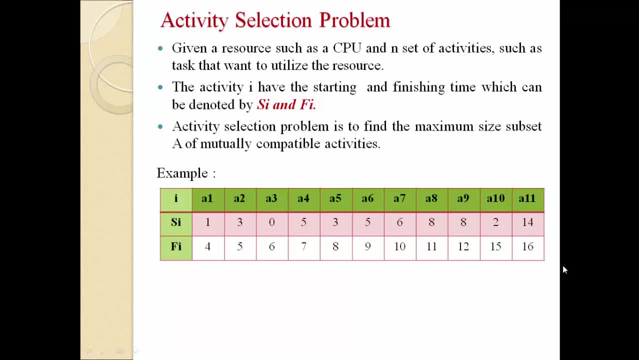 right. so now, uh, we have to identify the activity which is compatible. it means that we can execute all the activities in in. we have to identify the set which has a number of activities and all activities can be executed. so, as we discuss, we have only one cpu, so, at the time, only one activity can be executed and it is based on. 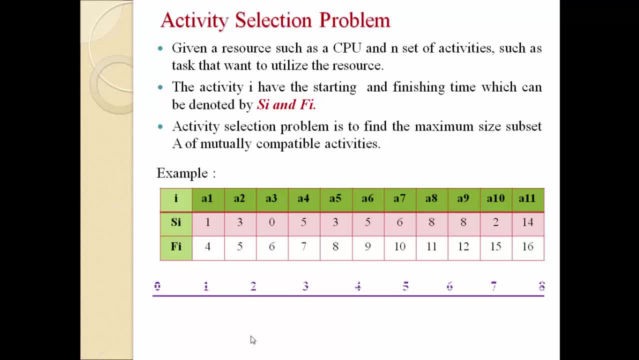 starting time and ending time. just take one example. suppose, uh, this is our timeline. we are starting from zero to a maximum value of our starting and finish time. we have to consider, for example, 16, then 0 to 16, uh timeline we have to set. but here i am just giving an example: uh, 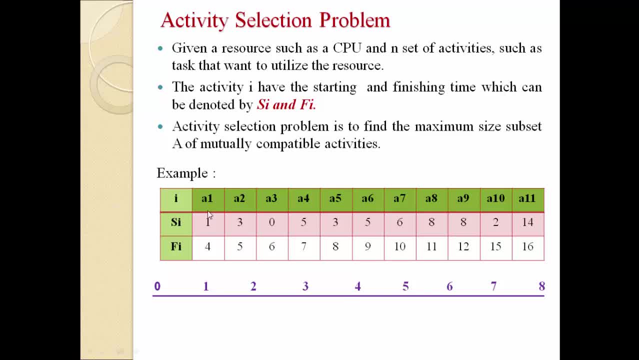 what is compatible activities are. so, for example, we are considering: a1 is our first activity, so starting time is one and ending time is four. so the activity a1 has a starting time one and ending time is suppose four. so now we cannot select any activities which has a ending, which has a starting time, uh, less than the four. it 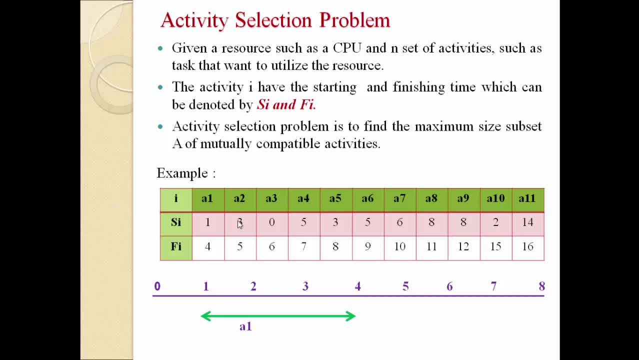 means that we cannot select a2 because a2 has a starting time three. at that time our a1, uh has a cpu. it means that a1 is running so we cannot choose a2 because it has a starting time uh, three and four, and a3 is a and our a1. so if we use cpu, so we can put a cpu the moment you run a cpu. 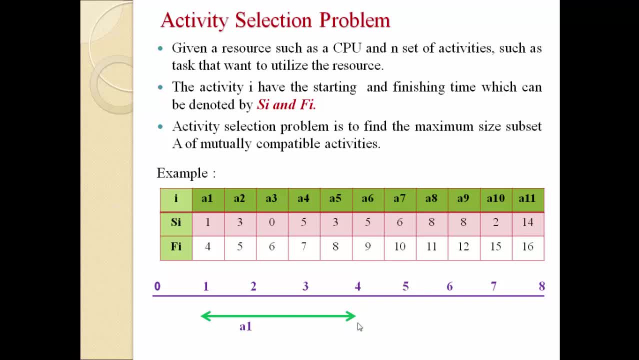 think so. we have to identify the activity uh which has a starting time either four or more than four, and this kind of activity is known as compatible activity. so identify a next activity which has a starting time either four or more than four. so a4 is compatible because a4 has. 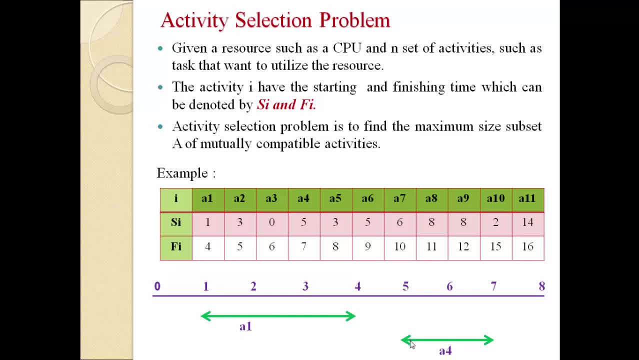 starting time five and ending time is seven. starting time five and ending time is seven. so a4 is than the four or equal to four. so it is greater than the four. so a4 is activity. so a4 is compatible. sorry, so, uh, in this way we have to identify set of activity, uh which is compatible. it means that 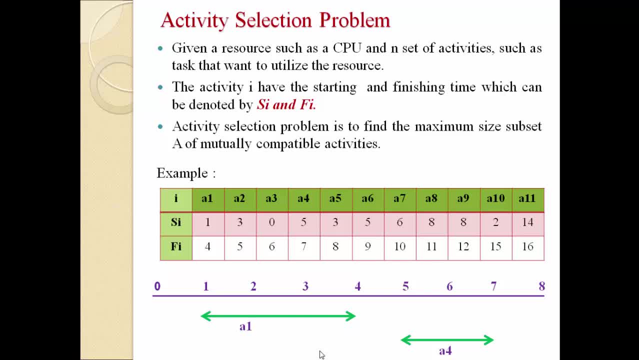 the second activity. uh, starting time of second activity must be more than the uh, more than or equal to the ending time of our first activity, right? so in this way we have to check and we have to identify different activities and we have to store in one set, and this set is known as solution. 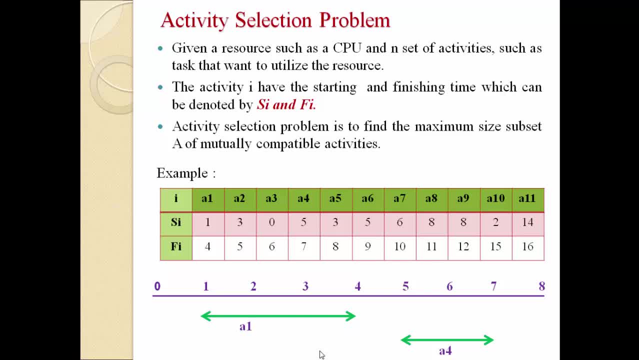 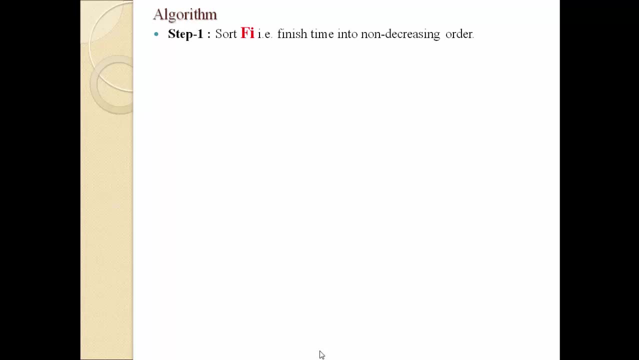 set. so let us solve this example so that you can easily understand every uh, every steps, how we can solve uh activity selection problem by using 3d method. so let us discuss algorithm. algorithm is nothing but set of steps. we have the step number one is sort f i, that is the finish time of activity. i finish time into non-decay. 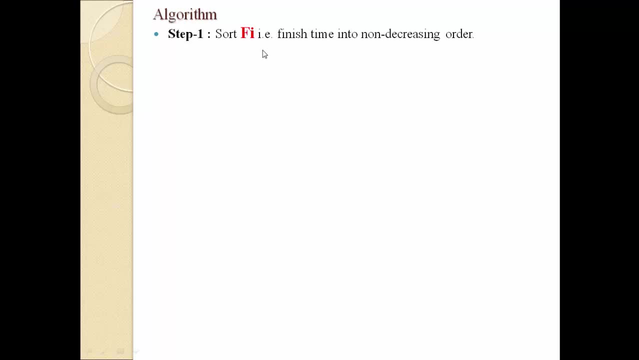 raising order. it means that ascending order. so we have to uh check finish time of every activity and we have to sort all the activities based on the finish time and, yeah, the we have to sort into the ascending order. step number two: select the next activity. i to the solution set, uh, if i. 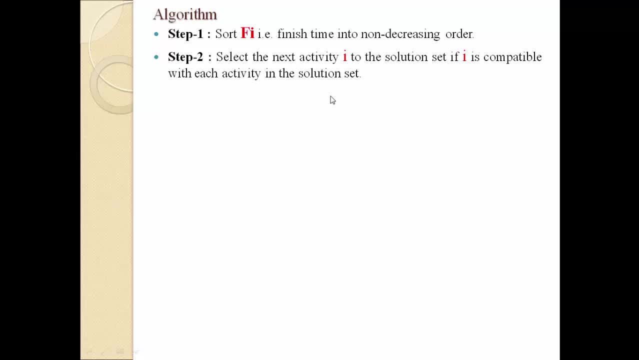 is compatible with each activity in the solution set. so, as we discuss compatible means, what the starting time of our previous activity? so the starting time of our next activity must be either equal or more than the finish time of our previous activity. so, uh, we have to uh identify. 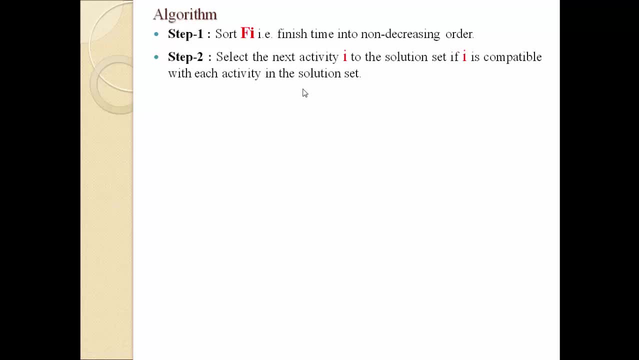 first activity, then find out the second compatible activity, then third compatible activity, like that and store in one set- step number three. repeat step number two until all the activities get examined right. so we have to start from the first activity to the last activity, identify all the compatible activity and store inside the one set right. this 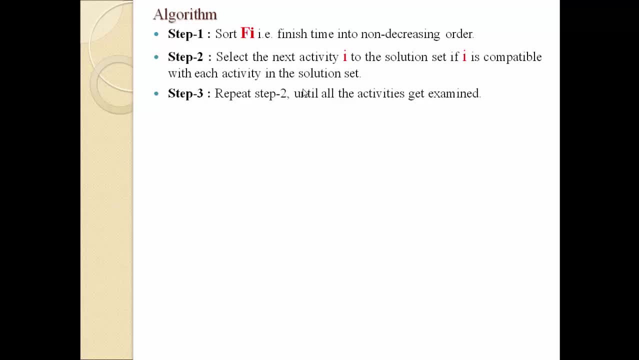 Algorithm is known as greedy algorithm, to find the solution of activity selection problem. Let's take our previous example, same. We are solving by using this all the steps. For example, we have a set of activities starting from 1 to 11. It means 11 total activities are there every activity has. 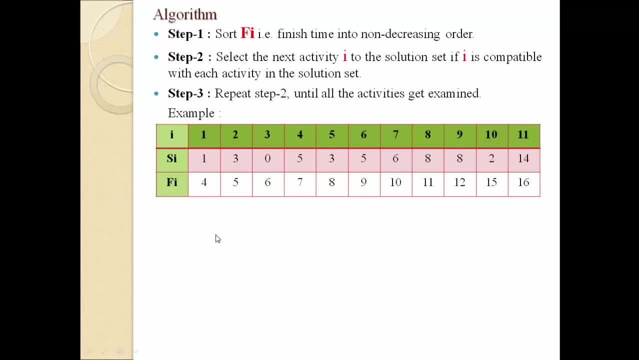 Starting, fixed starting time and a fixed finish time. that is ending time. Now step number one says that sort F I finish time into non decreasing order. so we have to check a finish time of all activity and we have to Sort into the ascending order based on the finish time of all the activities. 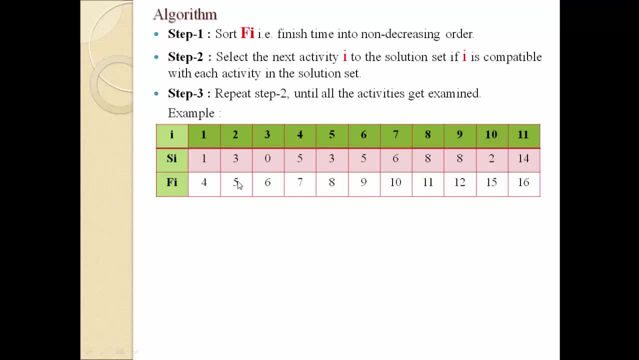 Just check. for example, one has a ending time for two as a five, three as a six, then seven, eight. So already it is in ascending order. suppose It is not in ascending order, then we have to sort first all the activities based on ascending order, based on the finish time. 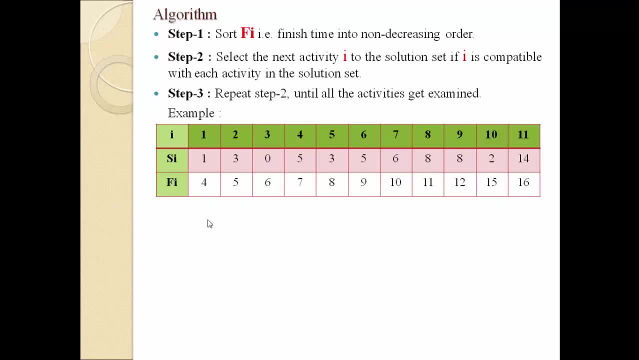 This is the step number one. again I am repeating: First step is we have to arrange all the activities based on the finish time and we have to sort all the activities in Ascending order based on the finish time. So once we check here the finish time of first activity, second activity, It is already in ascending order, So no need to. 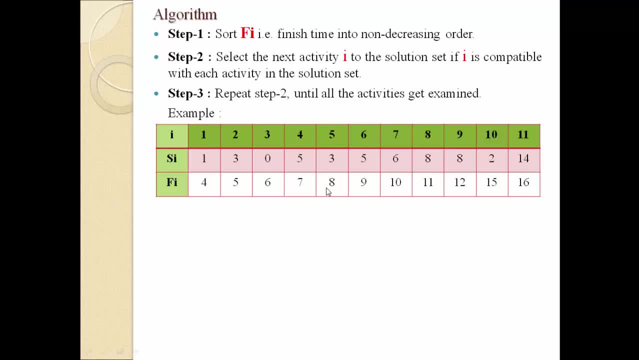 sort all the activities in ascending order. Now step number two says that we have to identify the Compatible activity first. First we have to select first activity directly and then find out compatible activity. We have to examine all the activities starting from 2,, 3,, 4 up to the 11.. 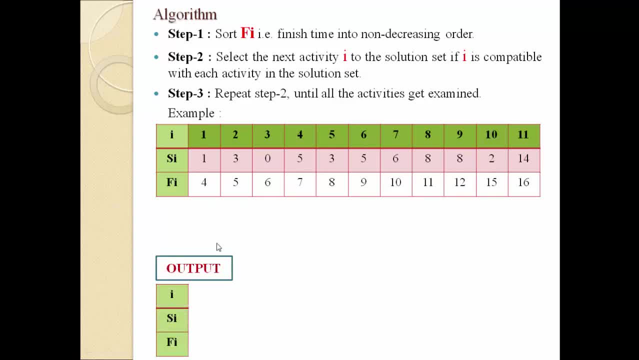 So let us start, Let us follow our second step. So here we will have output. Once we select any activity from this list, then we have to store inside this table, inside this set. So, as we discussed, we have already converted into ascending order. 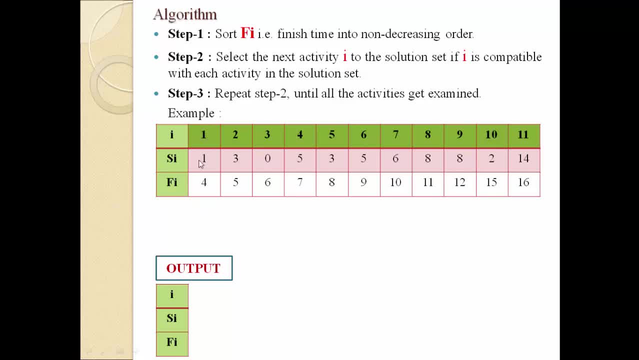 So first we have to select first activity directly, which has a starting time one and ending time four. So select first activity and store inside the solution set. We already selected our first activity. Then examine our second activity, which has a starting time three and ending time is five. 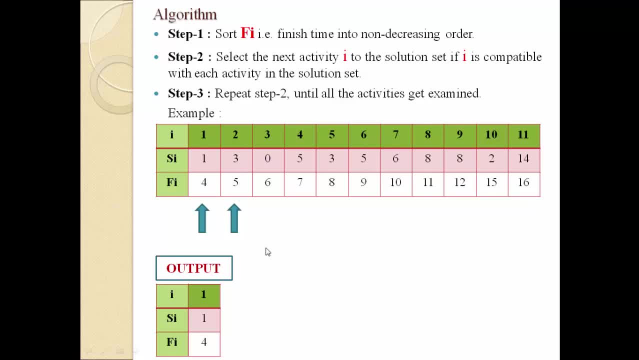 So, as we discuss your activities, only compatible if the starting time of your activity, current activity, is the rather than or equal to the ending time of our previous activity. so the previous activity has an ending time. 4, so if the starting time is more than. 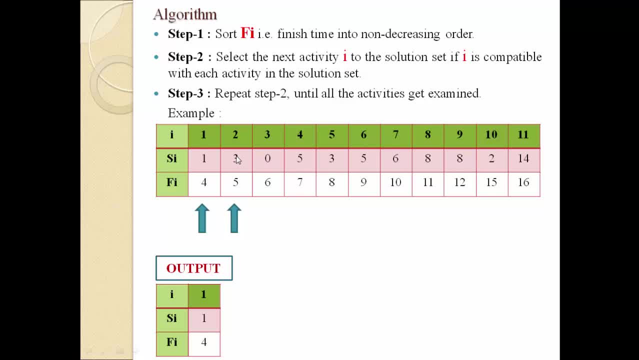 4 or equal to 4, at the time your activity is compatible, otherwise not. here the starting time is 3, so this activity is not compatible. now we have to examine our third activity, which has a starting time 0, so definitely it is also not compatible. then we have to examine activity number 4, which has a. 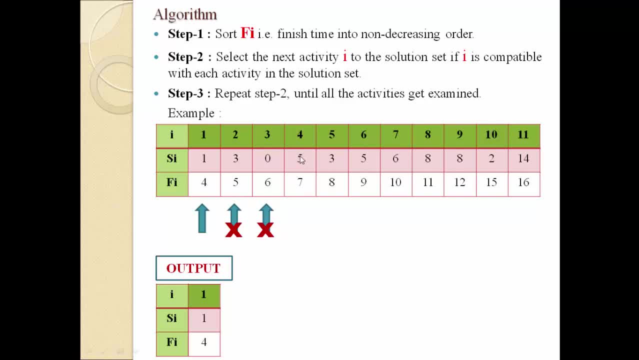 starting time 5, which is greater than or equal to 4. it means that it is greater than the 4, so this activity is compatible. so select this activity and store inside our solution set. so we are selecting activity number 4, which is compatible because the ending time is 4 and a starting time of fourth activity. 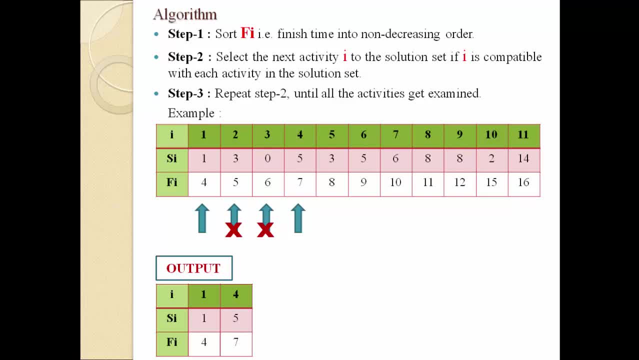 is 5, so this is compatible. now examine our next activity, which is the activity number 4, which is compatible because the next activity now we have to consider this activity as a current activity. this is our current activity, so we have to consider ending time. that is 7. so 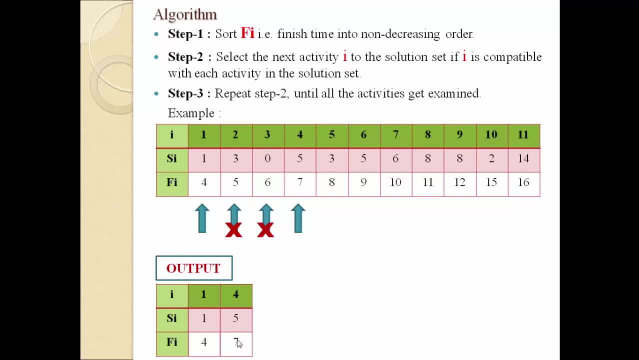 identify the activity which has a starting time either of 7 or more than 7. so just examine our second next activity, that is, activity number 5, which has a starting time 3. this starting time must be either 7 or more than 7, but it. 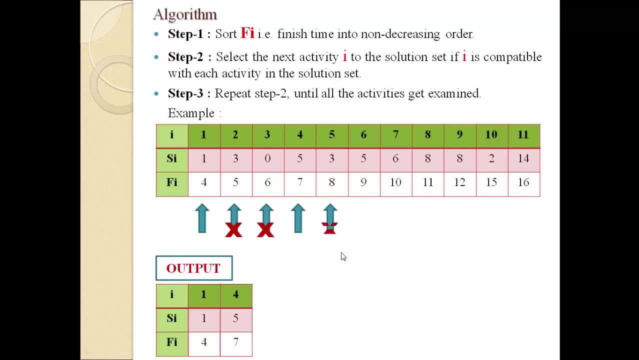 is less than the 7, so this activity is not compatible. then examine next activities. that is a 6 activity. number 6 has a starting time 5, which is less than the 7, so it is also not compatible. activity number 7, which has a starting time 6, so it is again not compatible. activity number 8: once we 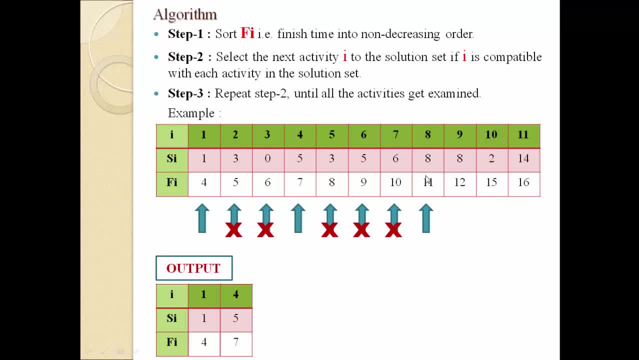 check the starting time of activity a number 8, then the starting time of activity number 8 is 8, which is greater than the 7. it means that this activity is compatible. so at this activity in our solution set and consider this activity as a current activity. so activity number 8 will be stored inside our solution set. 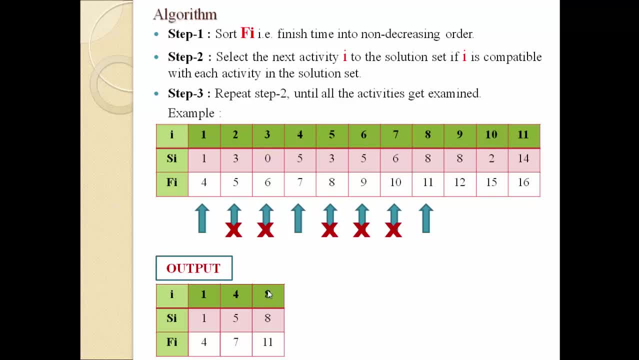 now, our current activity is 8 activity which has a ending time or a finish time that is 11. so we have to identify next activity which has a starting time more than the 11 or equal to 11. so our next activity, once we select, for example, 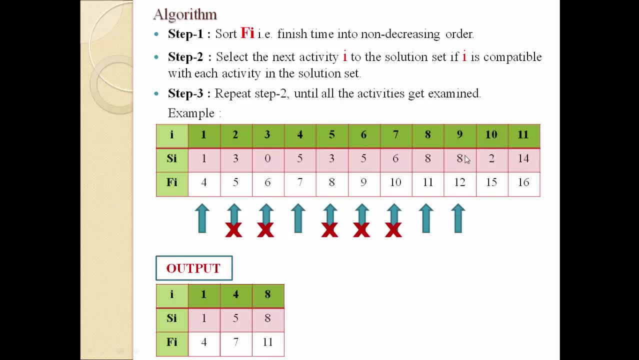 then it is our 9 activity, number 9, which has a starting time 8, so it is less than the 11. so it is not compatible. then activity number 10, which has a starting time 2, which is less than the 11, so again it is not compatible. last activity: 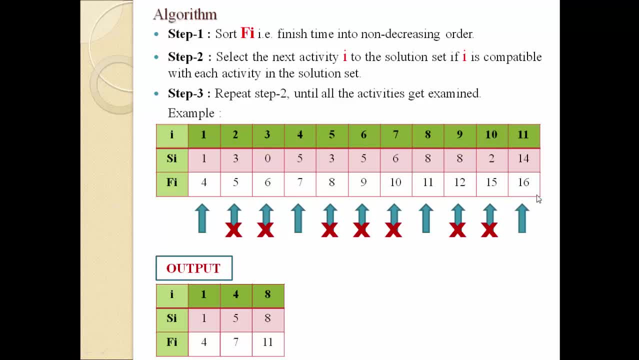 11th activity which has a starting time 14, so it is compatible and there we can select this activity because 14 is larger than the 11, so this is compatible and we can store in our solution set. so this is our solution now. there is no any other activity, so we have to. we have already examined all the 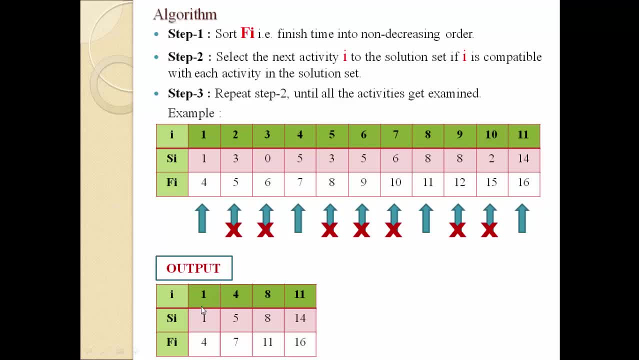 activities and we have a final solution set. we have selected activity number 1, 4, 8 and 11, so total 4 activities are there in this list, which is compatible, and this method is known as greedy method. so the final solution of our example is: we have selected total of 4 activity. that 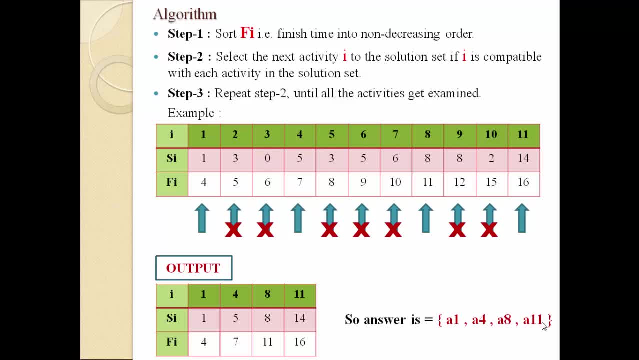 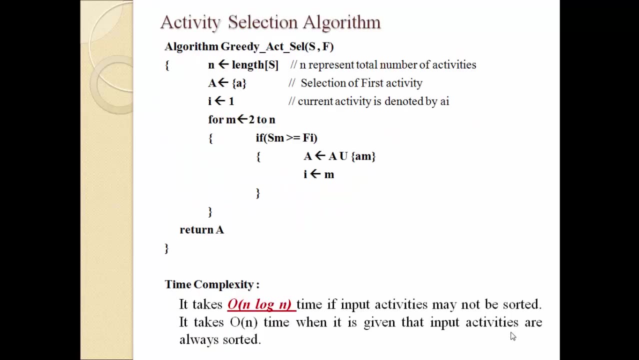 is a 1, elect activity, a 4, a 8 and a 11. these all are the compatible each other and this is the solution of our problem by using greedy method. now let us discuss a pseudo code of activity selection problem by using greedy method. in this pseudo code we are calling one function and name of the function is for. 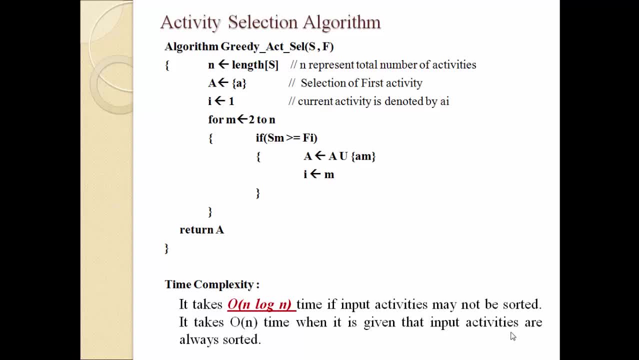 example, activity selection problem, in that we are passing two argument, S and F, if this is the starting time and ending time of all the activity. so the first step is we want to identify how many activities are there, so length of s we are finding to find how many activities are there, so, for example, small and 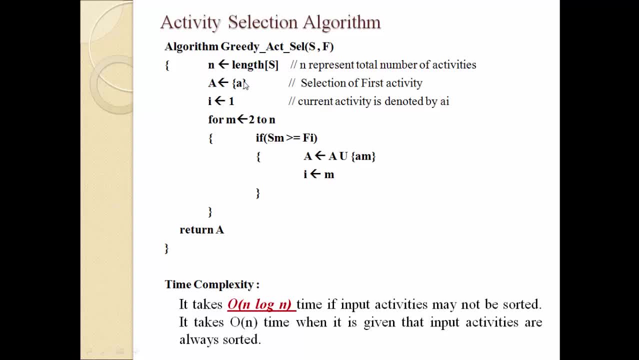 indicates number of activities. second step is we have to consider our first activities as a starting activity, because before that we have sorted all the activities into ascending order based on their ending time or we can say, finish time. so consider first activity and select it and store inside our solution set. that is our capital m, then i. 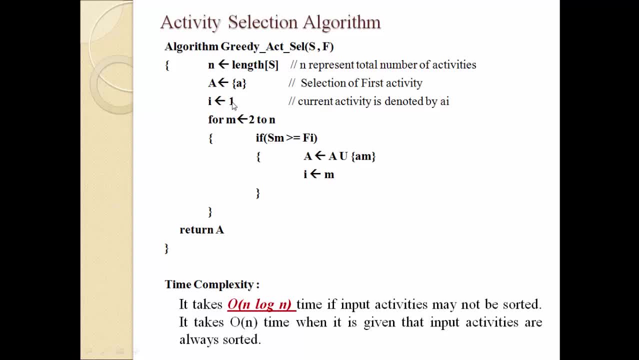 indicates our current activity. our current activity is equal to one. so first activity we are considering as a current activity. then, as we discuss, we have to examine, uh, all the activities. so we have to start from the second activity up to the last activity, that is, nth activity. 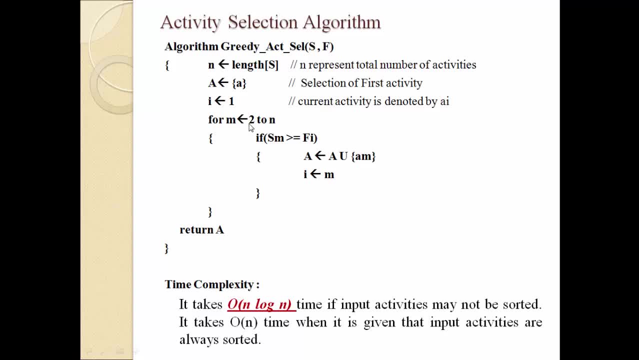 so this loop will be executed. uh, starting from m. m is equal to 2 to n, so it means that we have to examine all the activities. so every time we have to check that sm greater than or is equal to f? i. this f? i indicates finish time of our current activity. so when we select our next active, 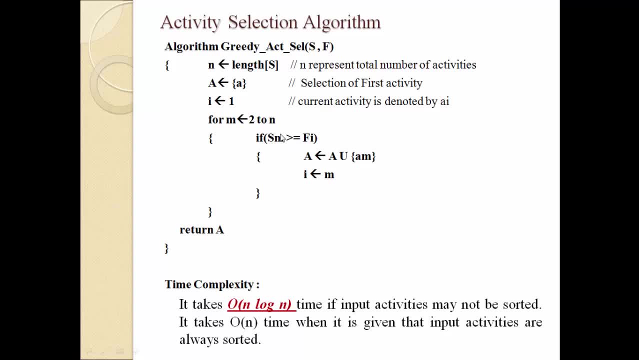 activity at that time. we have to check that, uh, the starting time of our next activity must be, uh, either greater than or equal to the finish time of our current activity. if this condition is true, it means that this activity is compatible and we have to store inside our solution set capital m, now this selected. 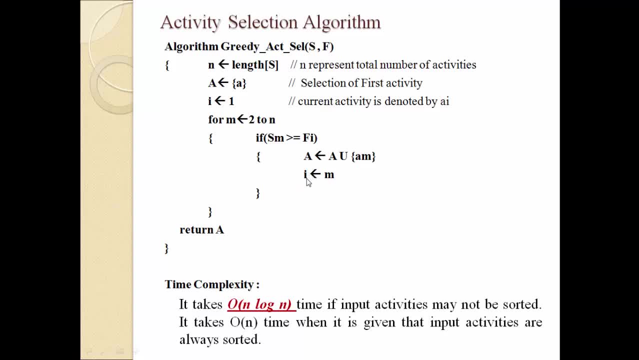 activity we have to consider as a current activity. so i is equal to m. so this loop will be executed, uh, until we examine all the activities. so this loop will be executed up to the end time. at the end we have to return our solution set, that is, our capital, m, once we uh check this whole algorithm. uh, or we can say all: 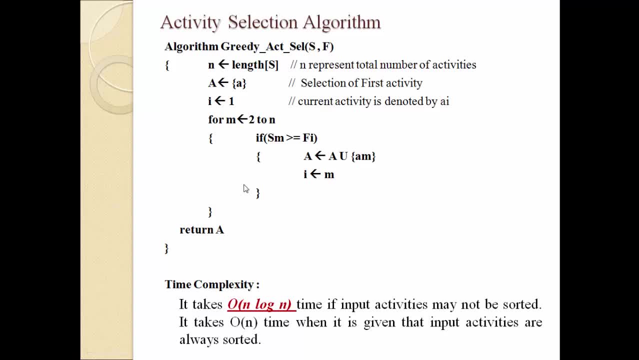 the steps of our degree algorithm at that time. uh, our second step size that we have to sort all the activities based on the finish time and must be sorted into ascending order. so, to sort all the activities into ascending order, we have a certain algorithm and, uh, the good algorithm we are. 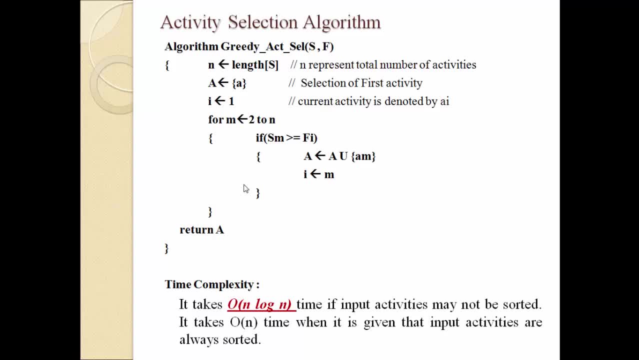 considering either the quickshot or merge sort, and both the algorithms are taking n into log n time, so we can say the maximum time to spend for this activity selection problem is sort all the activities into ascending order. then after we have only one loop to select all the activities, so this loop will be executed n times only.